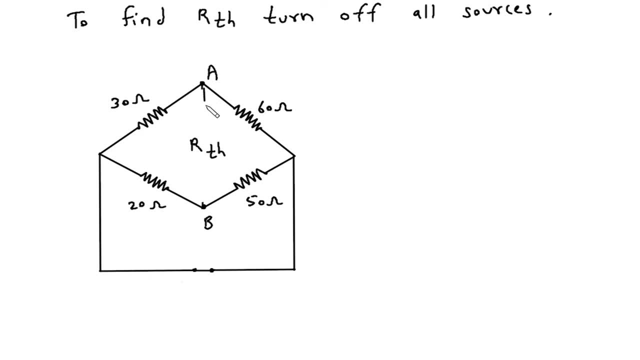 circuit when we turn off voltage source. Now here, this will be our RTH. Now here we can see that if we redraw this circuit, so it will be like: this will be A and this will be B. Now, if we stretch terminal A and B, it will be like this: If we stretch terminal A and B, 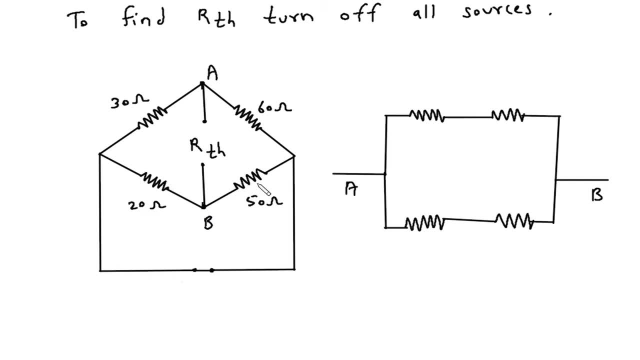 then this will be like this and also this will be like this: Now, if we stretch terminal A and B, these are connected like this. So here we can see, this is 60 ohm, 30 ohm. so this will be 60 ohm, 30 ohm, this will be 50 ohm, 50 ohm and 20 ohm. Now here we can see that. 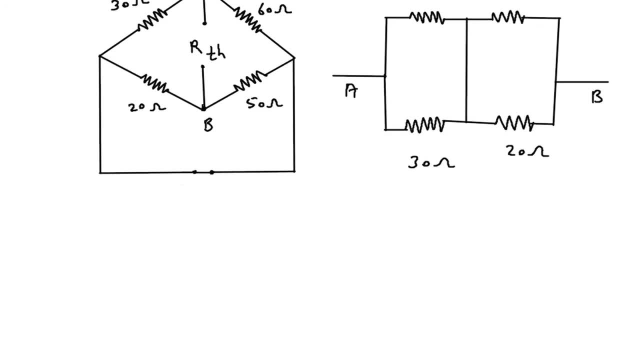 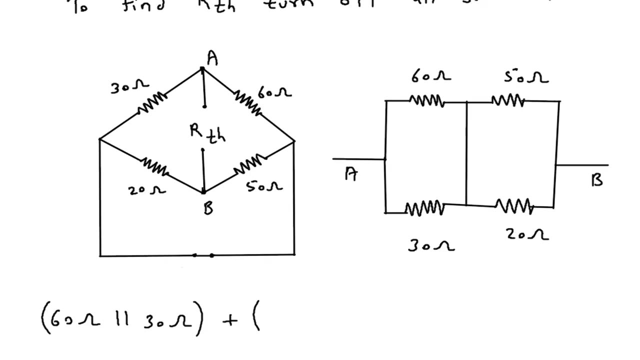 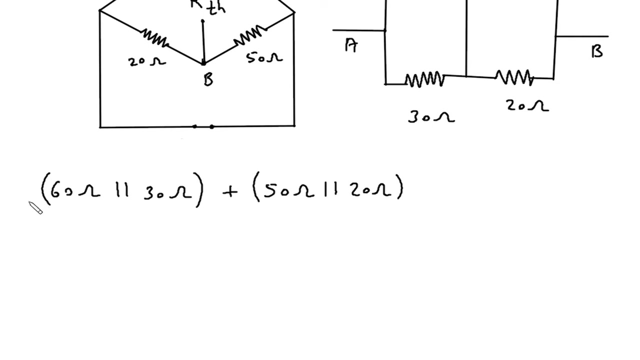 the 60ohm is in parallel with 30ohm, so 60ohm parallel with 30 ohm, and they are in series width: 50 ohm parallel with 20 ohm, 50ohm parallel with 20 ohm, so this will be 60 into 30 divided. 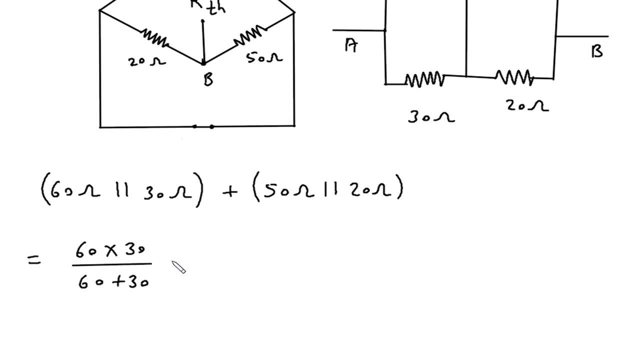 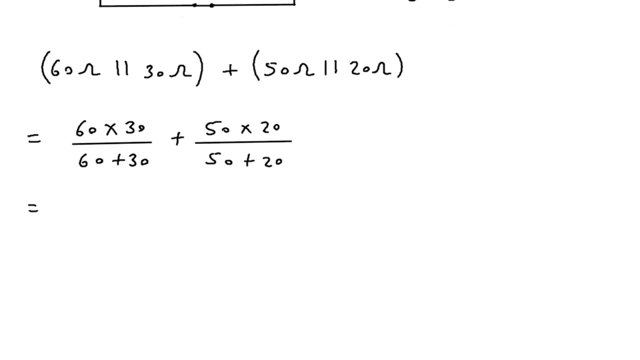 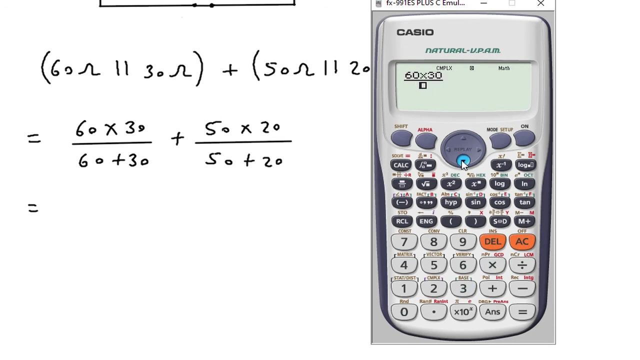 by 60 plus 30, then plus this will be 50 into 50 into 20 divided by 50 plus 20.. So 60 into 30 divided by 60 plus 30, then plus 50 into 20 divided by 50 plus 20.. 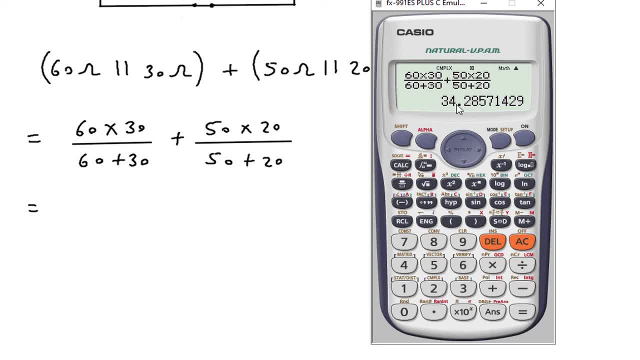 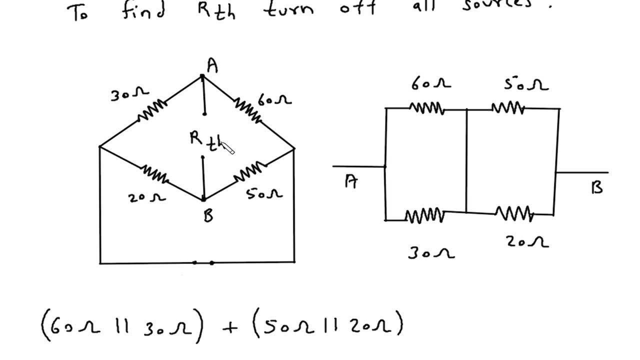 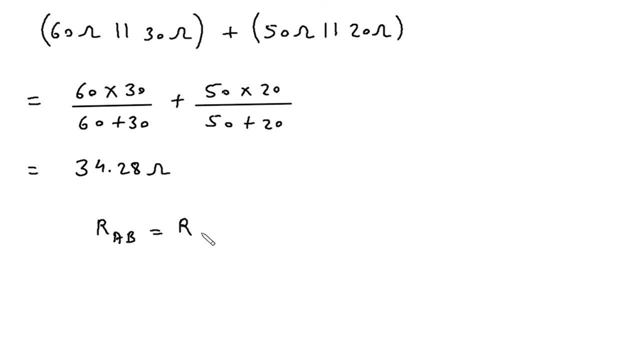 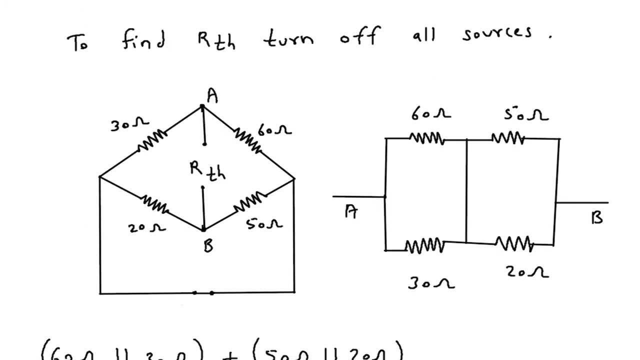 So it is 34.28 ohm. So therefore, RAB is equal to, RAB is equal to RTH, RAB is equal to RTH is equal to 34.28 ohm. This is the value for RTH. Now, next we have to find VTH. 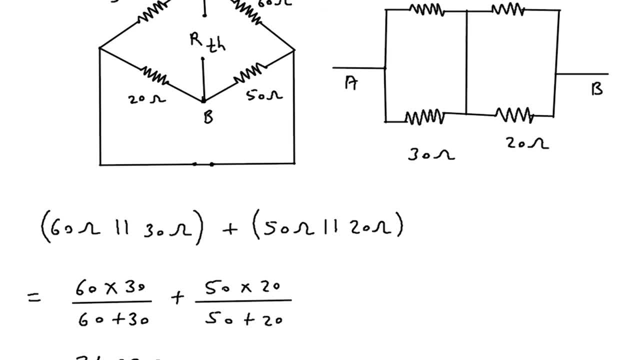 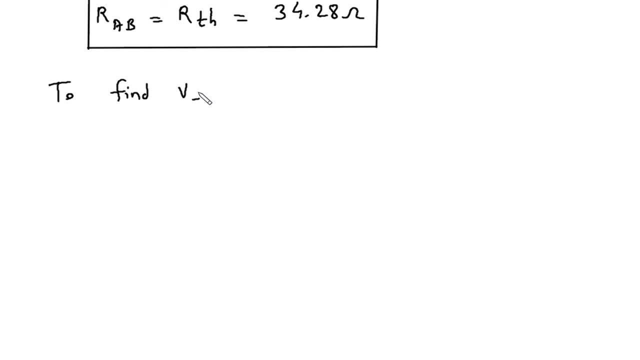 So to find VTH, that is Thevenin equivalent voltage, here this will be VTH, VTH, VTH, VTH, VTH, VTH. This is node A, This is node B, Let's say this is node C And this is node D. 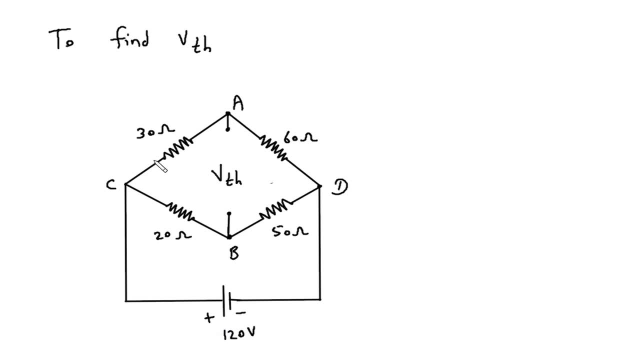 Now, according to the polarity of this voltage source, let's say, this is current i1 and this is current i2.. now, according to the direction of this current I1, this will be positive. this will be negative. now here, this will be positive and this will be negative. 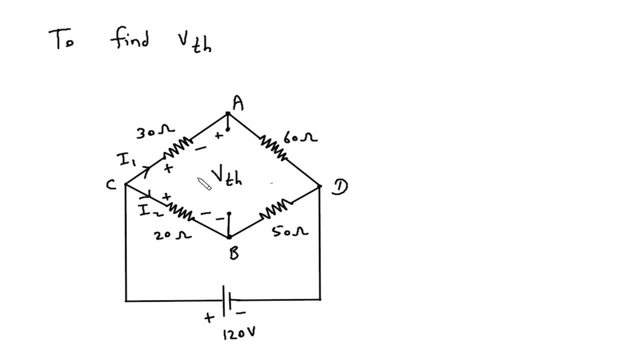 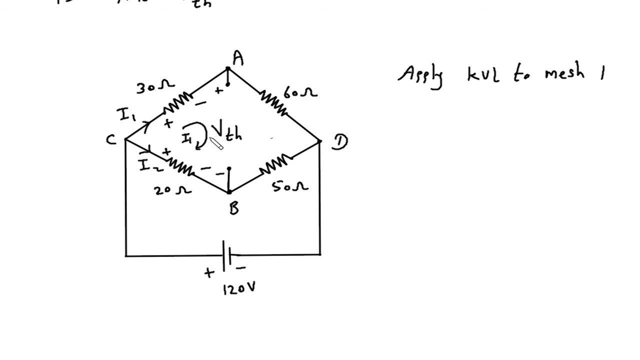 this will be positive and this will be negative. Now let's say this is mesh 1 with current, let's say, with current I1. Now we will apply KVL to mesh number 1.. Now, if we apply KVL to this mesh number 1, so let's say we will start from this point. so this will be. 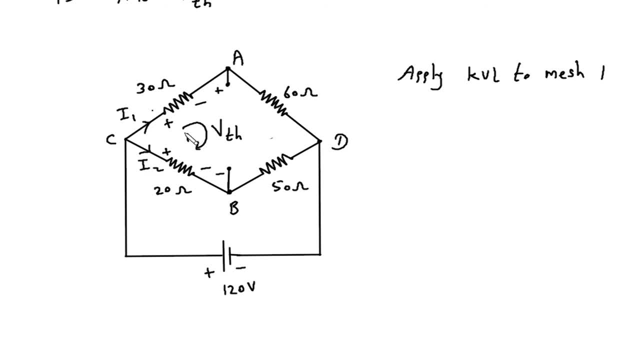 this is not current I1, this will be only mesh number 1.. Now if we apply KVL to mesh 1 and we start from here, so this will be plus 30 I1. so 30 I1 then plus Vth, plus Vth then minus 20 I2. 20 I2 is equal to zero. Now 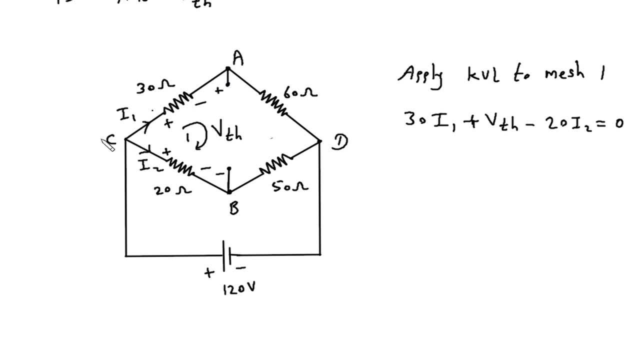 here we can see we need to find this current I1 first and this I2 to get the value of Vth. Now we can find I1, we can use here. voltage between this C and D will be same 120 V. so I1 is equal to V. by R, V will be same 120 because it is connected in parallel. so 120 divided. 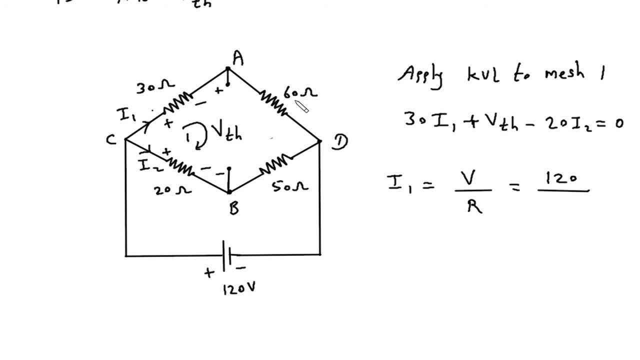 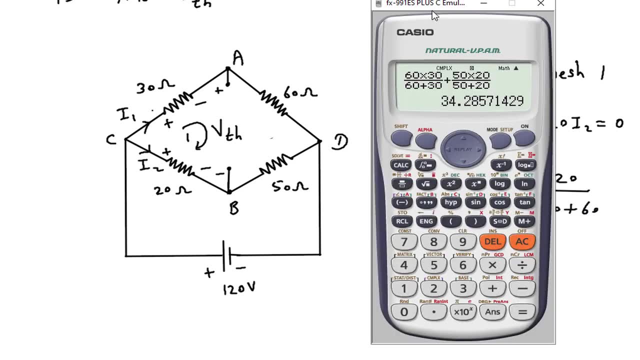 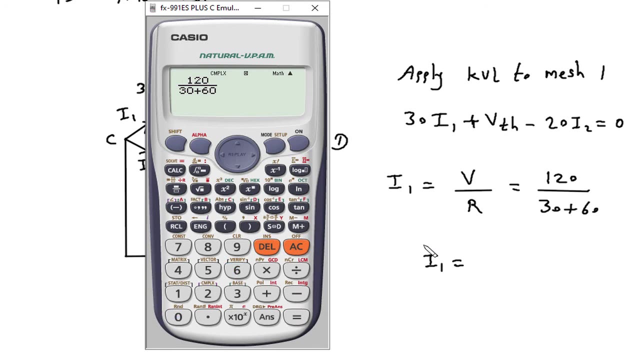 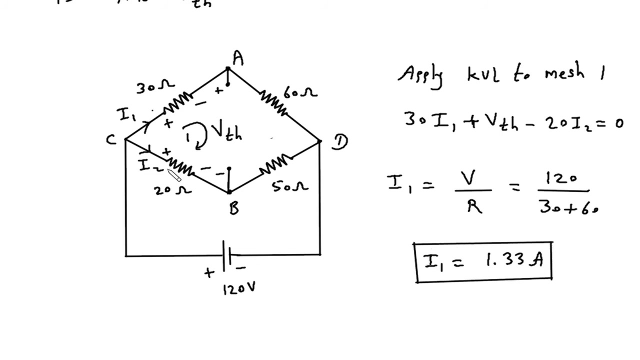 by R be 30 plus 60, 30 plus 60. So therefore I one is equal to 120 divided by 30 plus 60. So it is 1.33, 1.33 ampere. This is the value of i 1, then i 2.. Similarly we can find i: 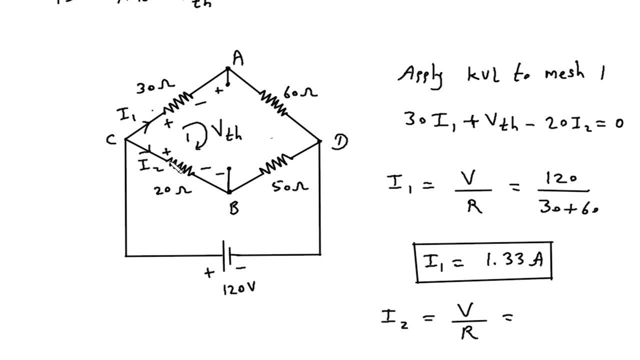 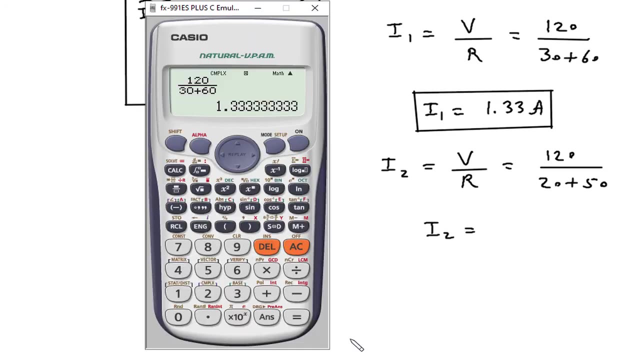 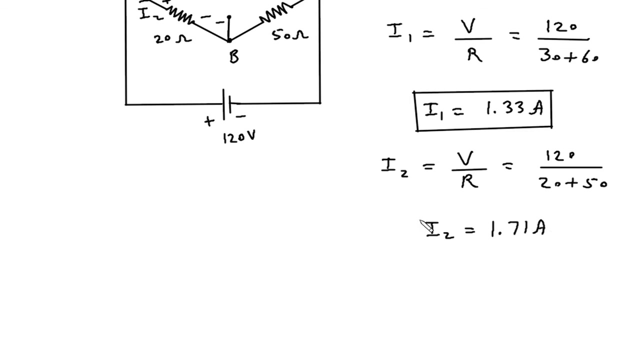 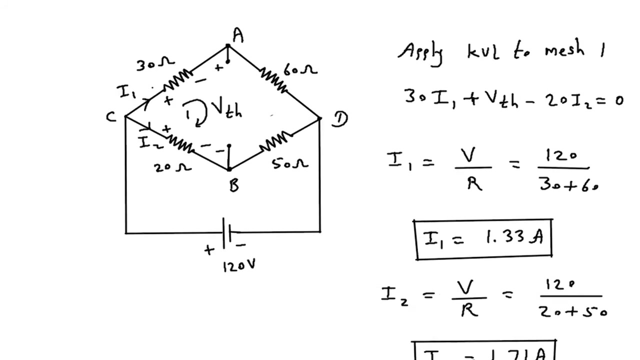 two by using v by r will be again same 120 divided by now here the resistance will be 20 plus 50. so 20 plus 50. So i is equal to 120 divided by 20 plus 50. so it is 1.71, 1.71 ampere. this is the value of I2.. 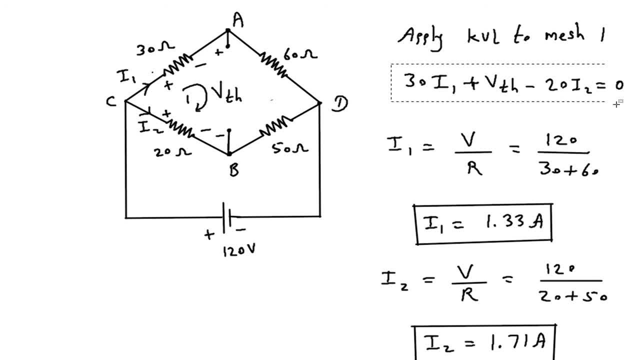 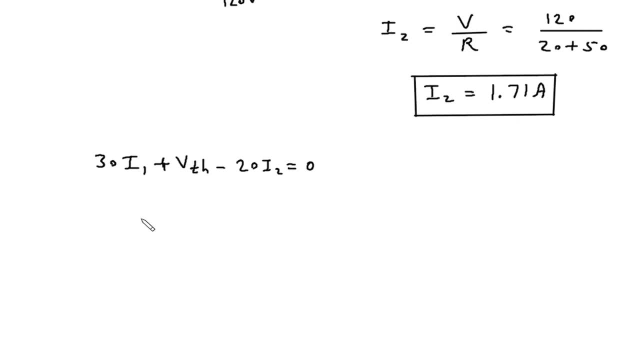 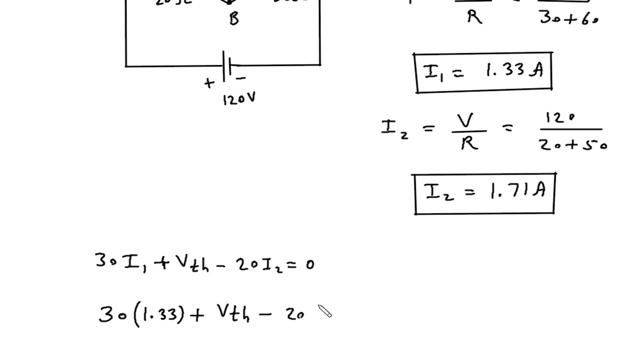 Now we can substitute this value here in this equation, so we can find the value of Vth. so this will be 30. the value of I1 is 1.33, then plus Vth, as it is minus 20 I2. now I2 is 1.71. 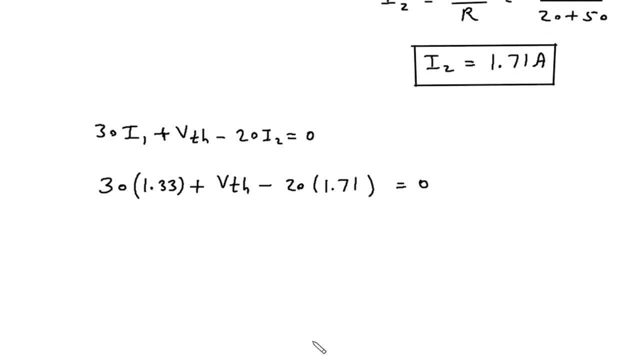 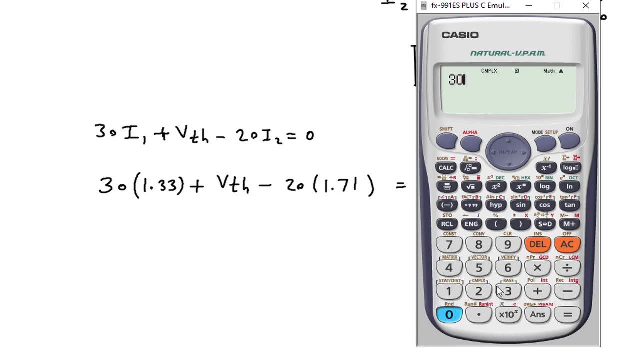 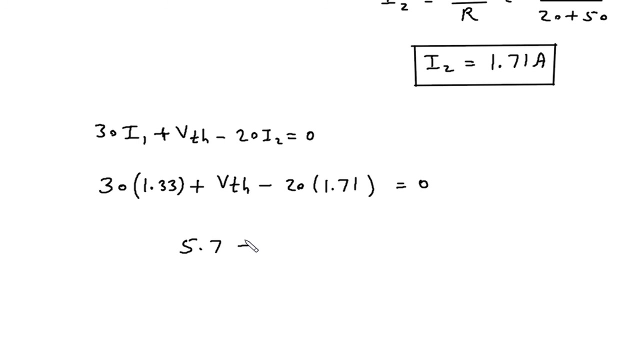 is equal to 0, so this will be 30: 30 into 1.33, then minus 20 into 1.71, 20 into 1.71, so this will be 5.7.. Ok, 5.7 plus Vth is equal to 0. now from this we can say: Vth is equal to minus 5.7 volt. so 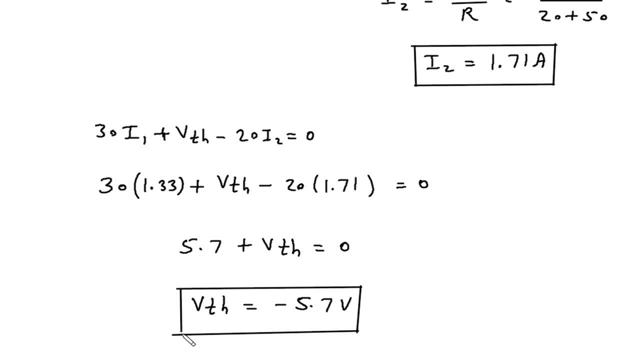 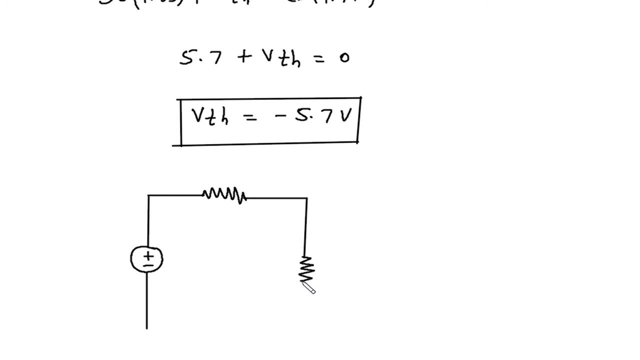 this is the value for Vth. now, from this values we can draw Thevenin equivalent circuit. so Thevenin equivalent circuit will be 30, this will be Vth and this will be Rth and this will be RL. now the value for this Vth. 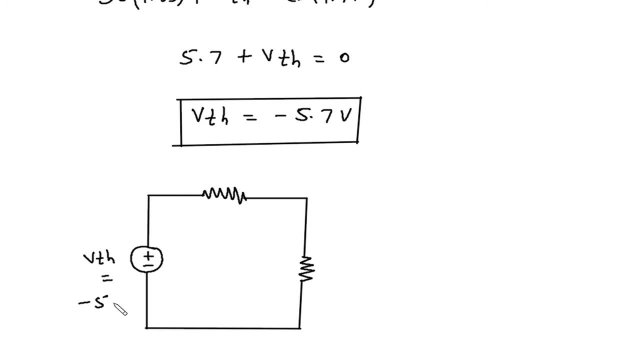 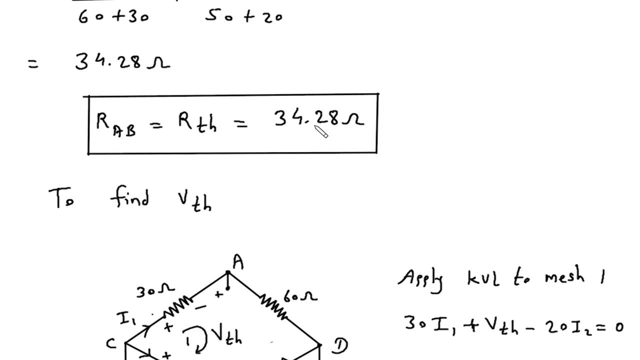 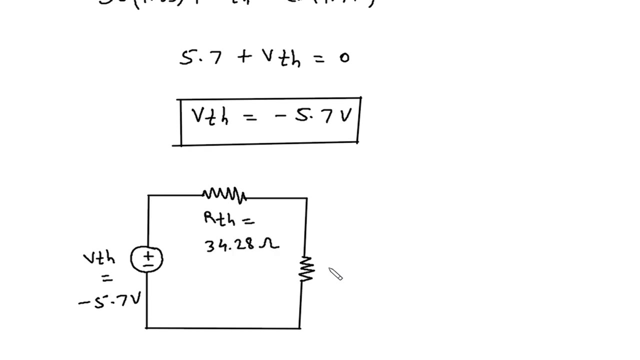 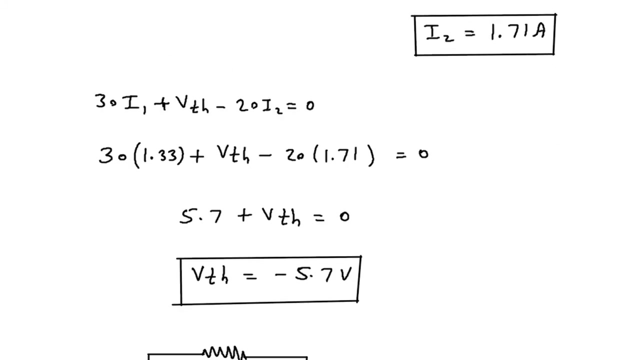 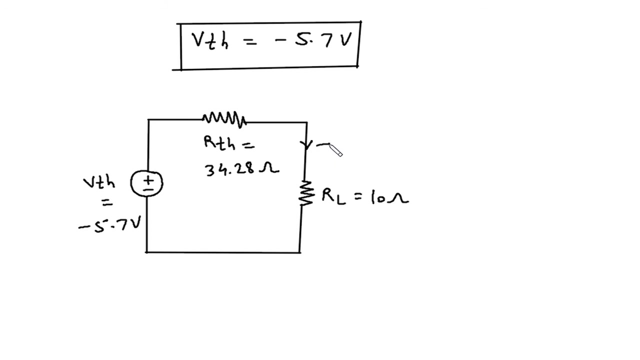 is Vth is equal to minus 5.7 volt. the value for Rth is 34.28 ohm. Ok, Ok, Ok, Ok, 34.28 ohm, and this will be RL, and RL is 10 ohm, 10 ohm and this will be IL. this will be. 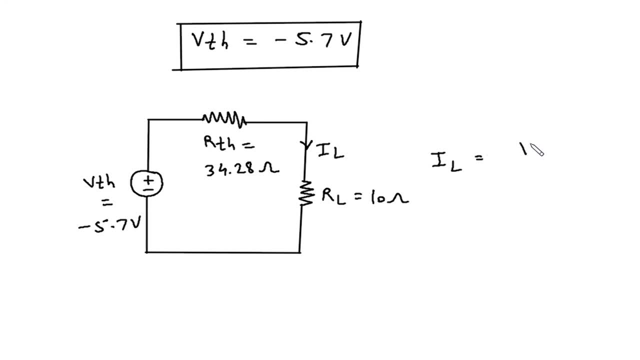 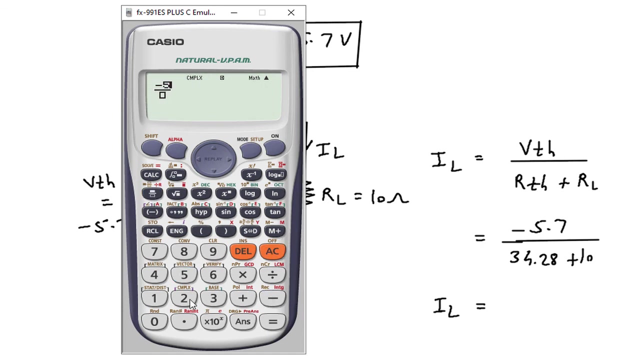 IL. Now we can find IL by using formula: Vth divided by Rth plus RL. Ok, Ok. Ok Now. Vth is minus 5.7 divided by 34.28 plus 10, so therefore il is equal to minus 5.7 divided. 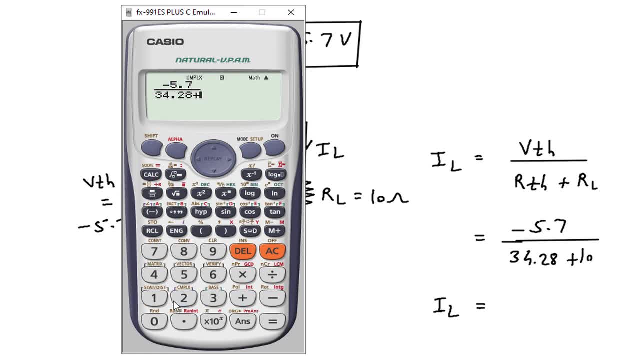 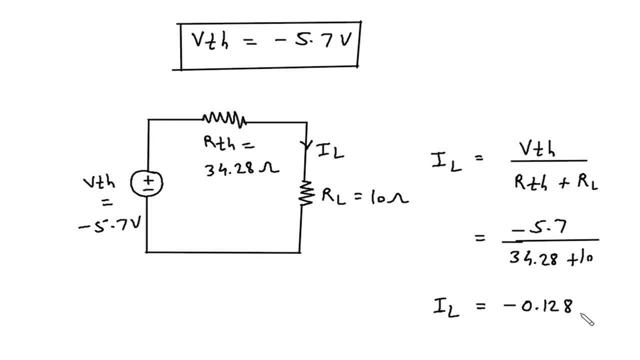 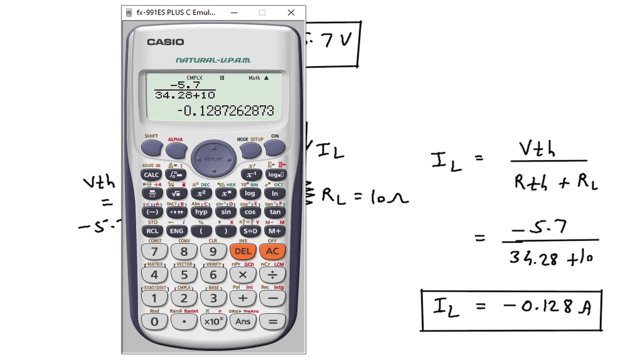 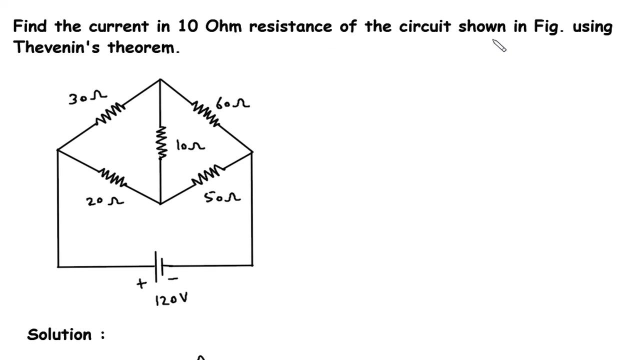 by 34.28 plus 10. so it is minus 0.128, minus 0.128 ampere. this is the value for il. what we have to find, we have to find: find the current in 10 ohm resistance of the circuit shown.